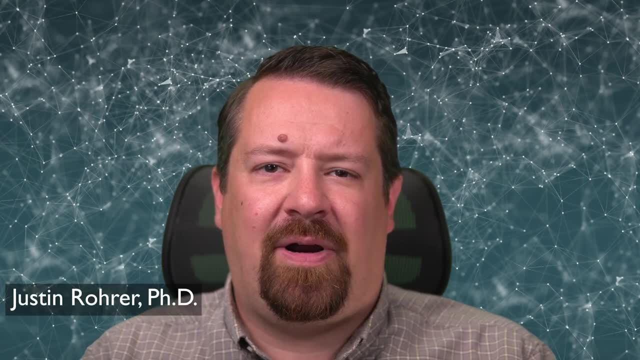 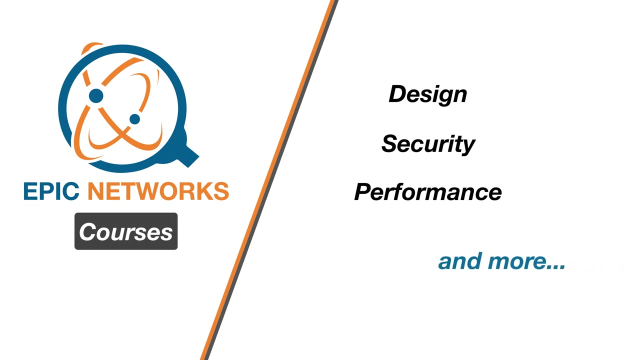 Welcome back. In this video, we're looking at operational security using firewalls and intrusion detection systems. Within firewalls, we'll look at both stateful and stateless packet filtering, as well as application gateways. Let's get started. In this video, we'll be looking at operational security, meaning firewalls and intrusion. 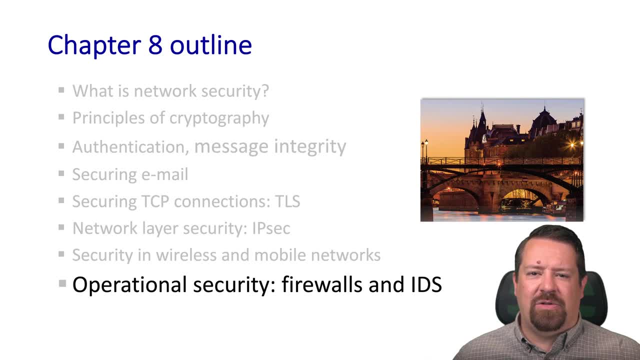 detection systems. The name for these devices that we've used previously in the course is middleboxes: Devices that look at multiple layers across the network stack, even though they sit out in the middle of the network. Statistically speaking, middleboxes in modern networks are nearly as 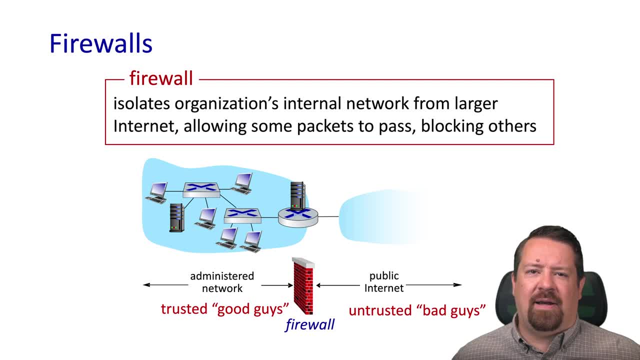 common as routers. A firewall is the name for a middlebox that isolates our internal organization's network from the larger public internet, and it determines that some packets should pass through and others should be blocked. Usually, there is a concept that those on the 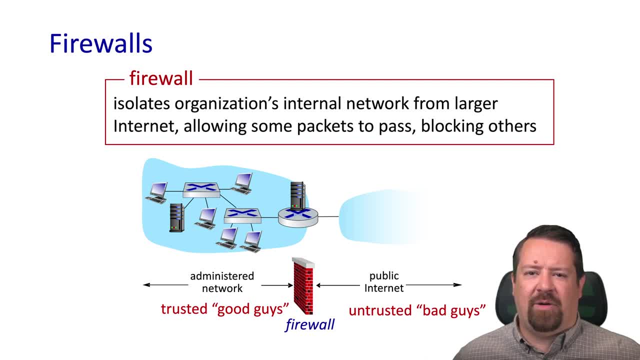 inside of the network are trusted and those outside the firewall are untrusted. So what are some of the things that we'll be looking at in this video? Let's get started First. let's talk about the attacks that firewalls try to prevent. A common one is denial of service. 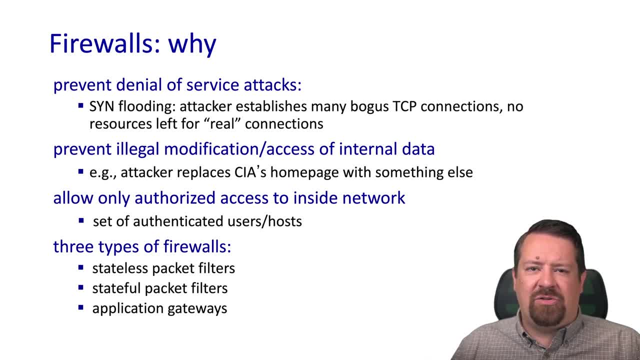 attacks, An attacker sending floods of SYN messages or other messages designed to tie up resources on the victim host. There are also supports to prevent illegal access to internal data, so protecting intellectual property of some form. It could also protect things like the public face of the company, where a hacker is trying to replace parts of the webpage, either to deface it. 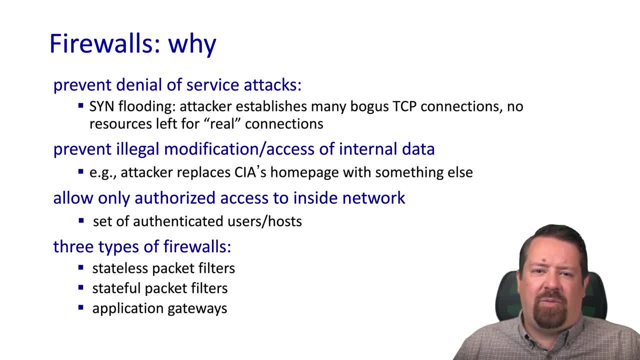 or to use it for some nefarious purpose. And we can break firewalls down into three categories: Stateless packet filters, stateful packet filters and application gateways. These are roughly in order of complexity where, as you go down that list, the mechanisms of the 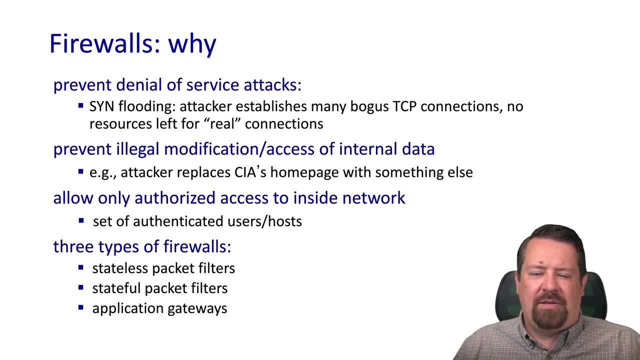 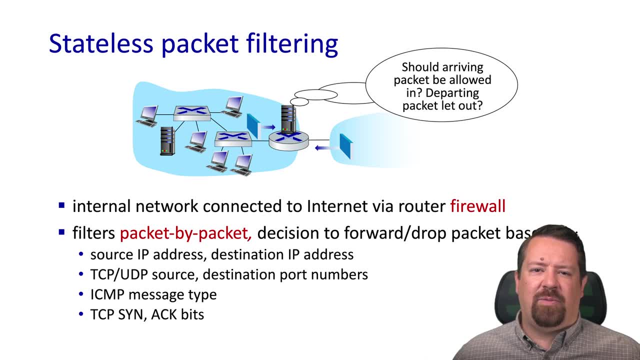 firewall become more complicated and more CPU intensive and may also have a greater impact on the performance of the network. So our first case is stateless packet filtering. These are where rules can be applied packet by packet and they make the decision to forward or drop a packet based. 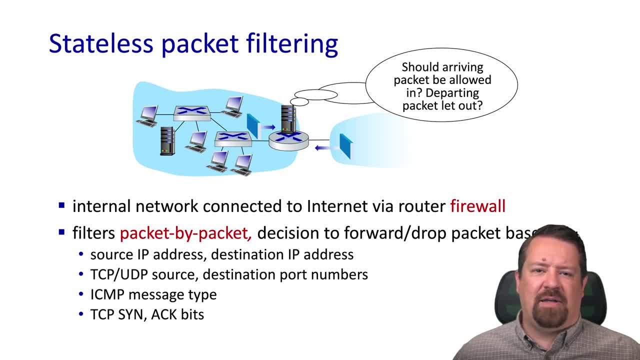 only on the properties of that individual packet, Things like the source and destination, IP address, TCP and UDP source and destination, port numbers, ICP, message types and TCP flags. So this is the most primitive type of firewall and, while it will catch many issues and block unauthorized traffic, 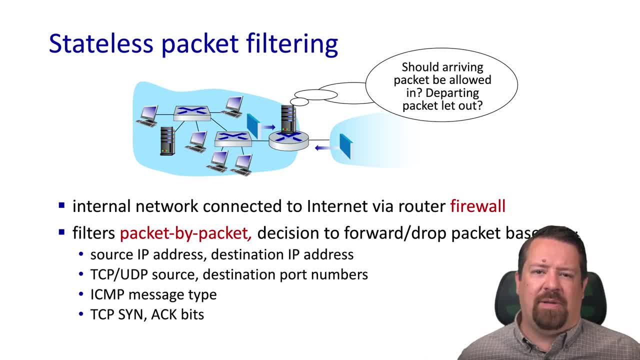 there are also things that it can't do, and we'll see that when we look at the more complex types. So, for example, a firewall might be configured with a rule to block incoming and outgoing datagrams that are using TCP source and destination port numbers. So, for example, a firewall might be: 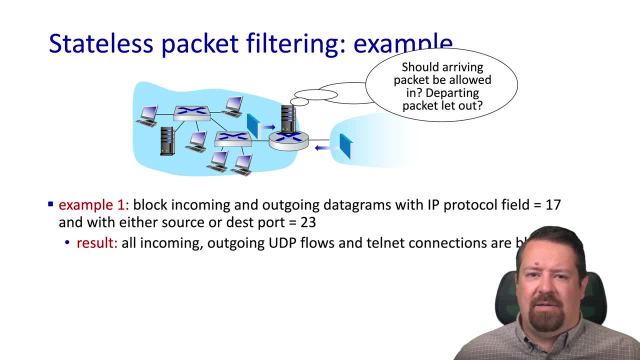 source or destination port 23. This is telnet, and many organizations block telnet because usernames and passwords are transmitted in the clear and so they don't want their users inadvertently using telnet to a remote site and sending out a password which might or might not. 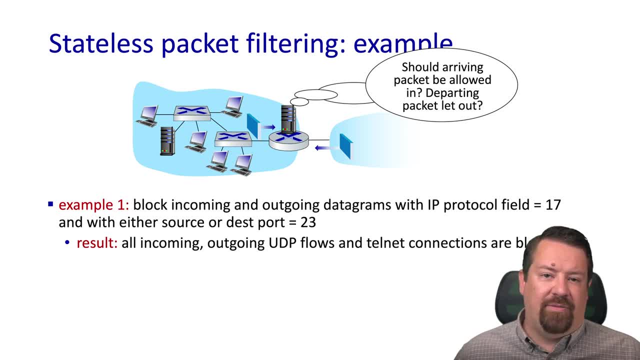 be the same as a password that's important to this entity, or revealing even the username. We also see that there's a rule in this firewall blocking IP protocol, field 17,, which is the UDP protocol. So this firewall is also going to block all UDP datagrams And, of course, the most common application to use UDP is DNS. 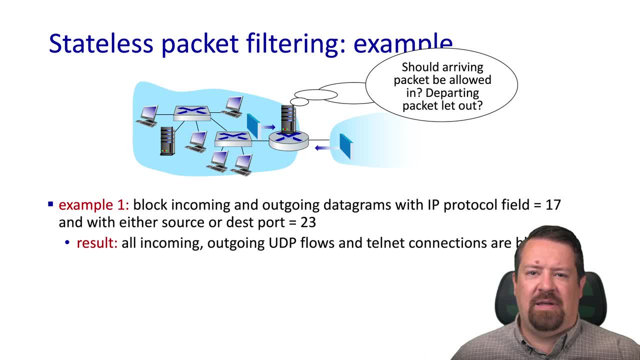 So this is preventing users inside this network from accessing DNS servers outside the network. another common security policy, Another example rule, might be to block inbound TCP segments with ACK equals zero, which is intended to prevent external clients from making TCP connections with internal clients, But it doesn't apply this on outbound TCP segments, so it wouldn't prevent. 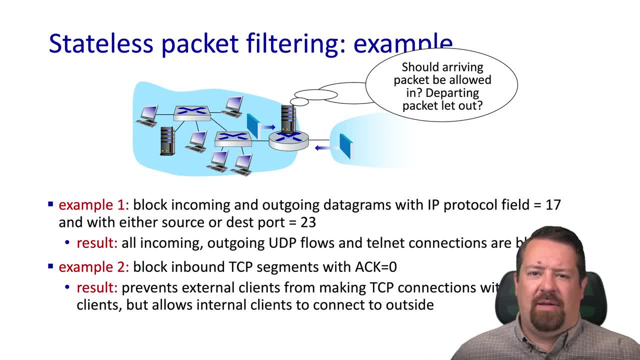 internal clients from connecting to the outbound TCP segments. So this is a rule that's going to not be very effective, and it might be better to look at the SYN flag and ACK flag and make a decision based on those. Here are some more examples of rules that we might use. 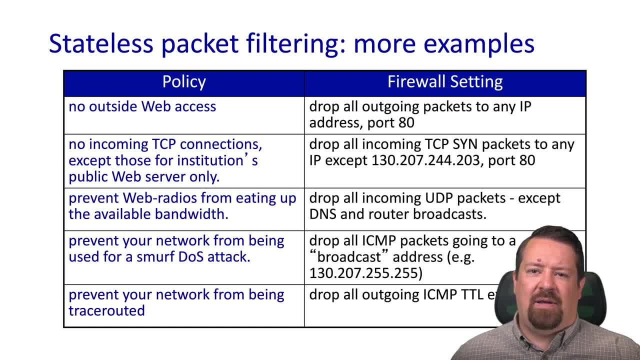 If we wanted a policy of no outside web access, then we could drop all the packets going to TCP port 80.. Of course, many websites are using HTTPS on port 443, so we would also have to those If we wanted to block incoming TCP connections. so new connection establishments. 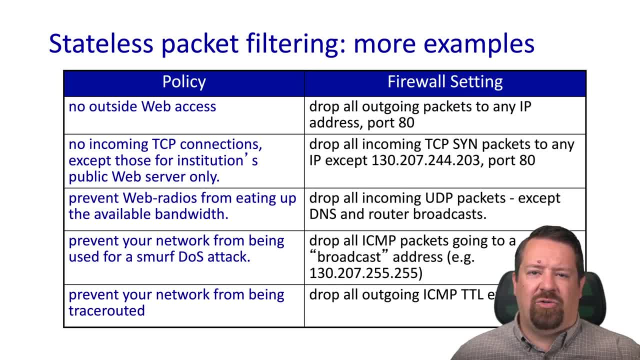 except those headed for the web server. we could have a rule that says: drop all incoming TCP SINs except for specific web server IP address and port numbers. We might want to block web radios by blocking UDP packets, although most streaming media have migrated to run over HTTP, so that's. 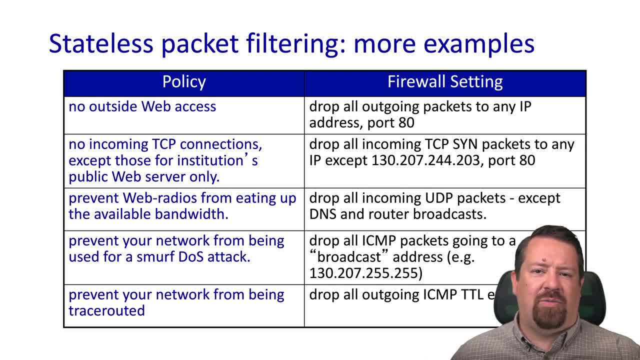 probably not going to block much And, as we see, in that case, if we wanted to still allow DNS, we would have to explicitly permit that. Another policy might be to prevent the institutional network from being used as part of a Smurf DOS attack, which could be done by dropping all. 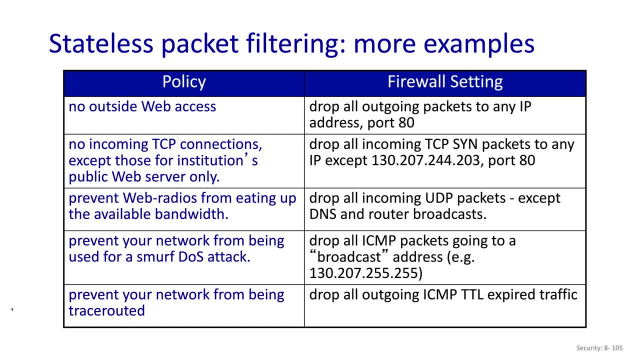 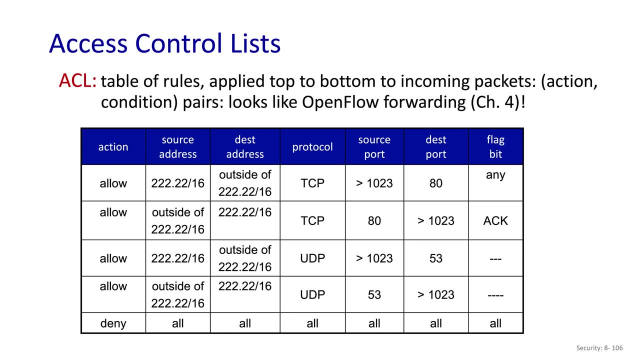 ICP packets going to a broadcast address, And our last example is to break traceroute, and this can be done by dropping all outgoing ICMP TTL expired messages. So these rules are going to be implemented as a table, commonly referred to as an ACL, an access control list. 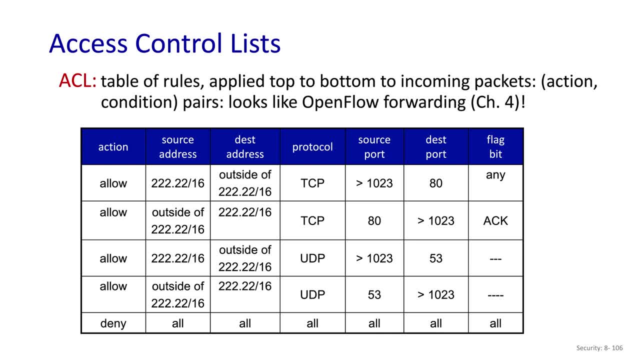 And I've been around forever, and this is essentially what OpenFlow forwarding decisions are based on, only with more fields available in the OpenFlow case. Now these rules are going to be applied in order, so the first one that matches is going to be applied to that packet and it will not see. 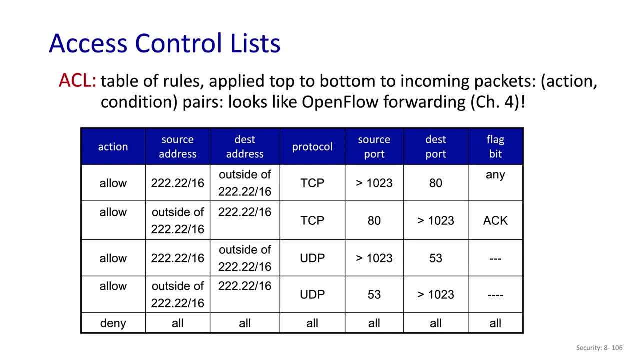 the rest of the table. So, for example, we're allowing any packet on this slash 16 address that's tested outside of that address where the protocol is TCP, the source port is an ephemeral port and the destination is 80. We're going to permit that. So these are outgoing. 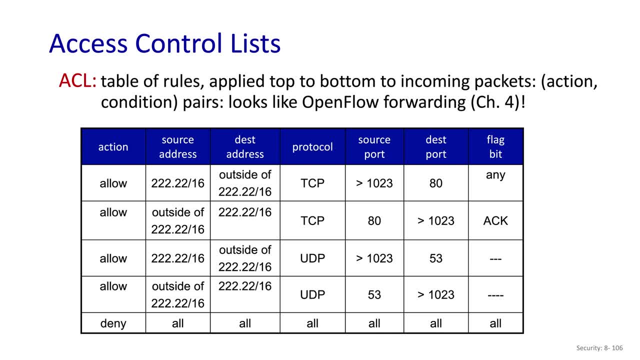 web traffic. And then we also have to allow the incoming web traffic, not new connections, but the responses to our outgoing connections. so we see that rule looks very similar, but reversed. So it's allowing sources outside of the network to contact destination addresses inside the network. 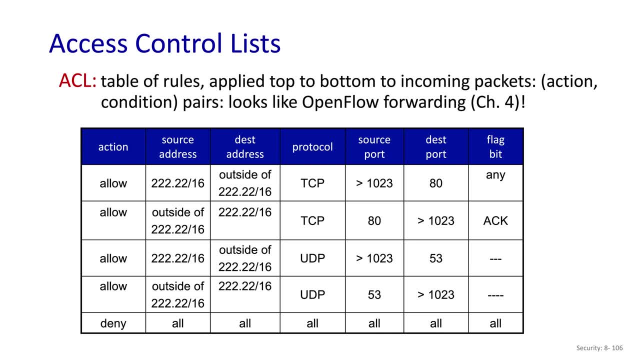 a protocol, TCP, where the source port is 80,, meaning it's coming from the web server and it's destined to an ephemeral port, and it has the ACK flag set. You're also allowing UDP on port 53,, so DNEA 53, and you also have the port 53, which is the same one as the ACK flag set. You're also allowing UDP on port 53, so DNEA 15,, and you're also allowing UDP and port 53, so DNEA 19.. You're also allowing UDP on port 53, so DNEA 20,, and you're also allowing UDP on port 53, so DNEA 12.. 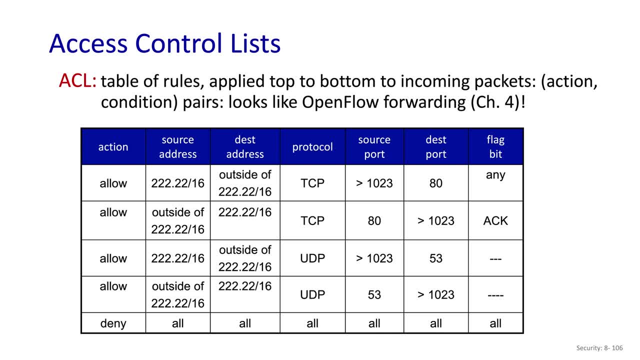 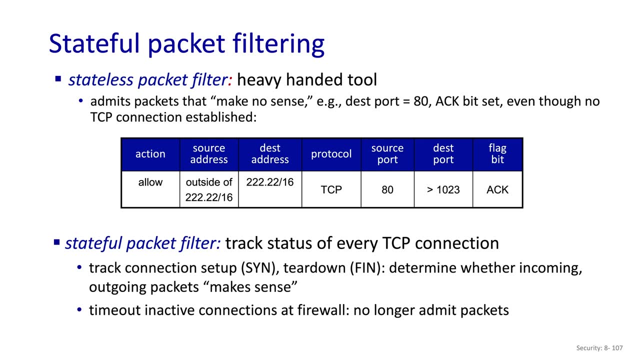 UDP on port 53. So DNS traffic and the responses, And then we're denying everything else. So it's common for an ACL to have an implicit deny at the bottom or an explicit deny rule. So here we get to the limitations of stateful packet filtering And it's primarily that the tool is not very. 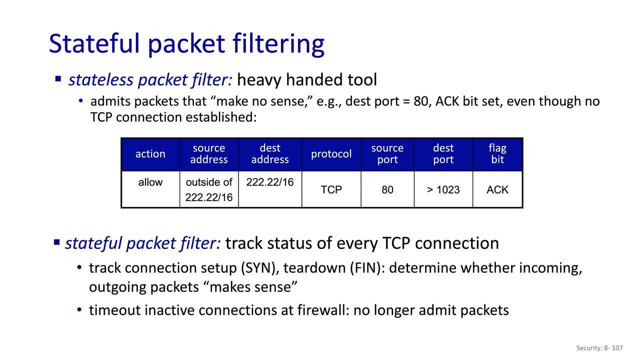 sophisticated, So there's still packets that can get through this rule set that don't make sense. For example, we're letting through these acknowledgements, but there might not be a corresponding connection established, So it might just be scanning traffic that's been sent out with. 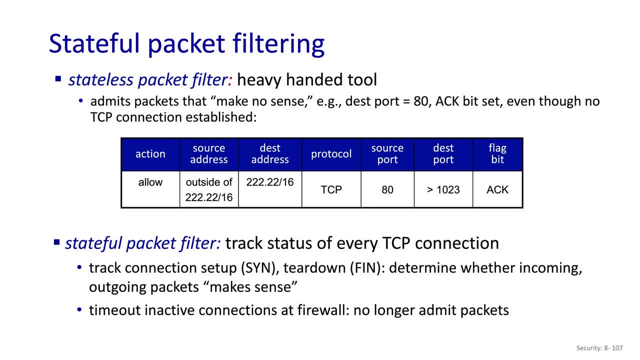 the ACBIT set. A stateful packet filter keeps track of the status of every TCP connection that's going through it. So it knows when the connection setup happens, when the teardown happens, So it can determine when to remove these connections from the state that is tracking. It knows whether it's 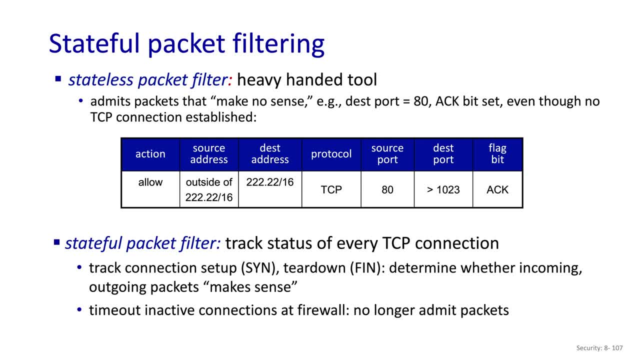 an incoming or outgoing connection. And so if a TCP packet comes along that doesn't match one of these existing sessions and is not a new connection setup, then it can drop those packets, even if they would otherwise match a rule and be allowed. The stateful packet filter can also time out inactive connections. So even if an explicit 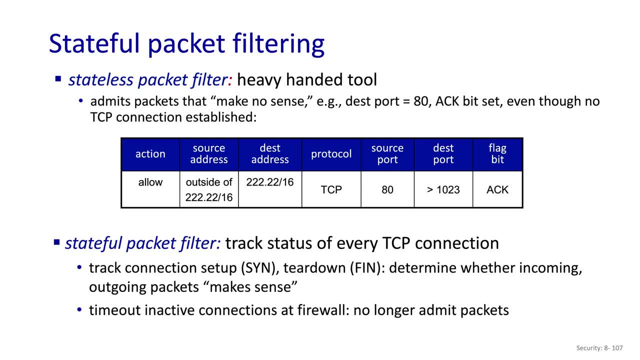 fin has not happened. the host on one end or the other might have disappeared, And so it can remove these from its table and no longer admit packets to them. Of course, you can cause lots of issues for your network with a stateful packet filter if this timeout is too aggressive such that long. 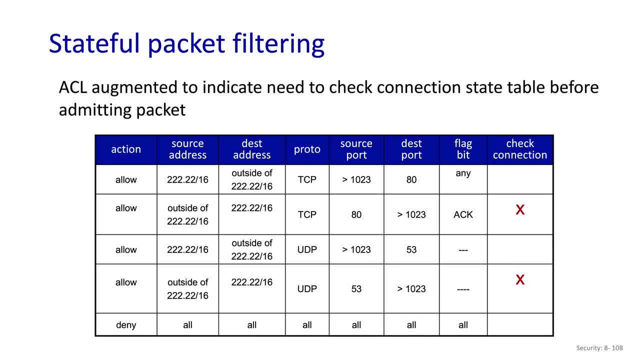 TCP sessions get broken by the fault. So if you have a stateful packet filter you can also check the firewall. So now in our stateful packet filter ACL list we have the same set of rules, But before allowing certain packets we're going to check that a connection exists. So in our first rule we're 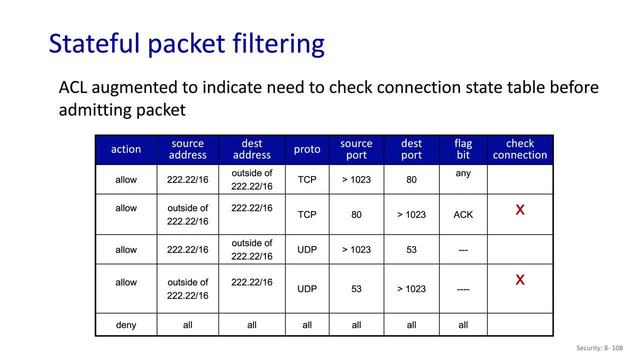 explicitly allowing setup request to happen, So there doesn't have to be an existing connection, because we want to allow the SYN through with this rule. However, in the second rule, we're only trying to allow AXE through, not any random packet, And so these packets should match existing. 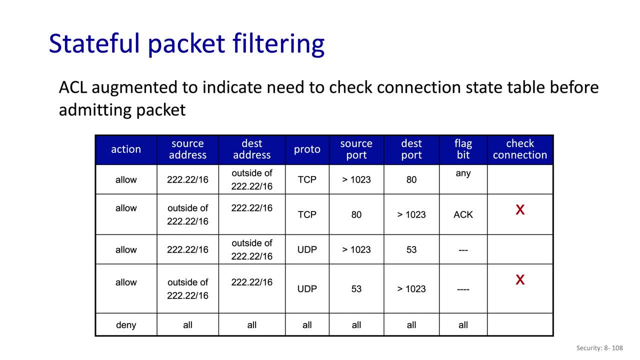 connections. So we're going to check it on the second rule, Likewise with the third rule. we're allowing for initial DNS requests to go out, but the response back should match an existing session at that point established by the outgoing request And if not, we're not going to allow those packets. 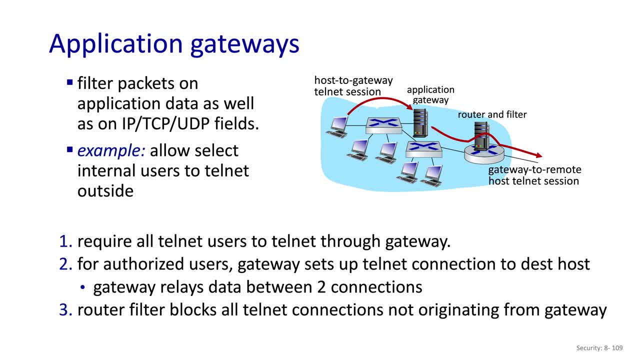 in All right. now we get to the most sophisticated version, which is the application gateway. So we can think of the stateful packet filter as operating at the transport level. It understands end-to-end flows and that there should be associations that packets belong to. 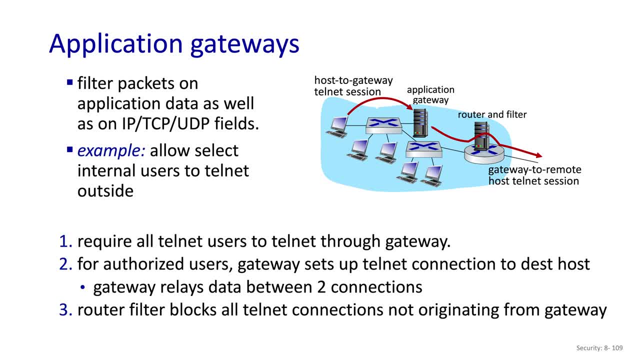 Application gateways go up another layer to the application itself and it understands how specific applications work and what should be allowed or not based on the rules of those application layer protocols. So in this example we want to allow some users to telnet outside. 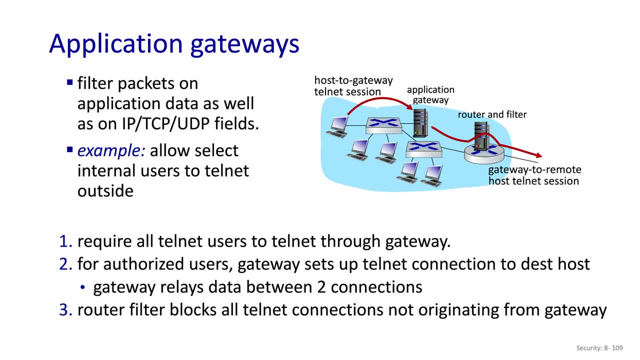 So it's going to require all the telnet users to telnet through a gateway Instead of telnetting directly to their outside address, which would be blocked by the firewall. they have to connect through the gateway And, if the user is authorized, the gateway sets up the telnet connection. 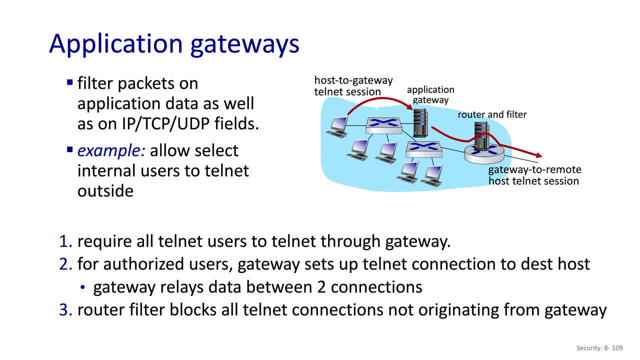 to the destination host. So this application gateway is always going to sit in the middle of the connection from a TCP perspective. The host established a TCP session with the application gateway. The application gateway established a new TCP session with the end destination And by the. 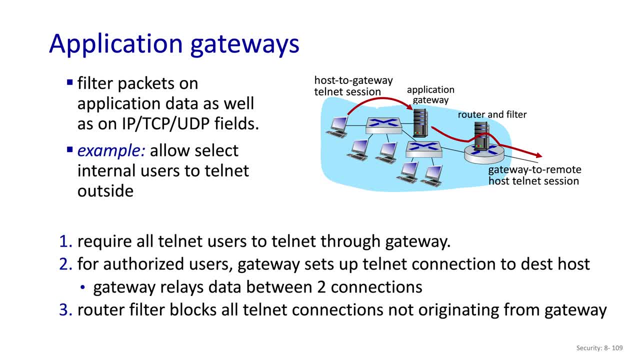 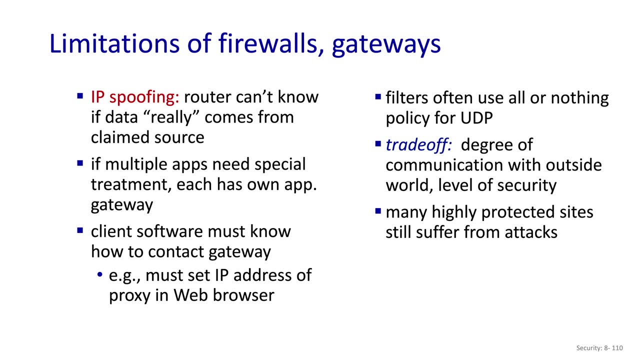 way, this application gateway has to be allowed through the firewall to get there. So the router blocks all telnet connections that didn't come from the gateway, which simplifies its rule set. All right, we have some limitations when dealing with firewalls and gateways. Number one is IP spoofing- IP addresses. 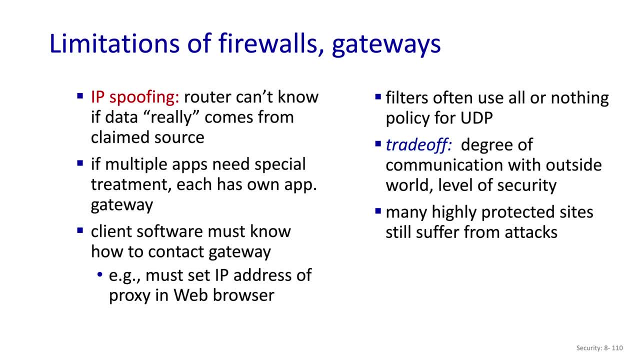 are not validated in any way, And so lots of entities on the internet or even on the local network could change the source IP address to someone else's and send out packets. Another limitation of application gateways is that you need one for each application that needs special. 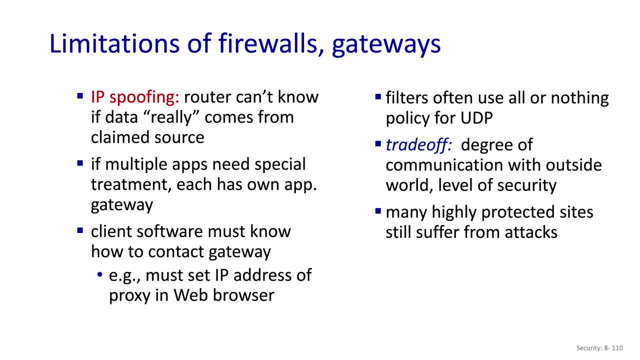 treatment. It's difficult for users to adopt a new application that needs to get through the firewall, And even the creation of an application gateway may lag far behind the popularity of a particular application itself. And then the client software for that particular application has to be able to configured to talk to an 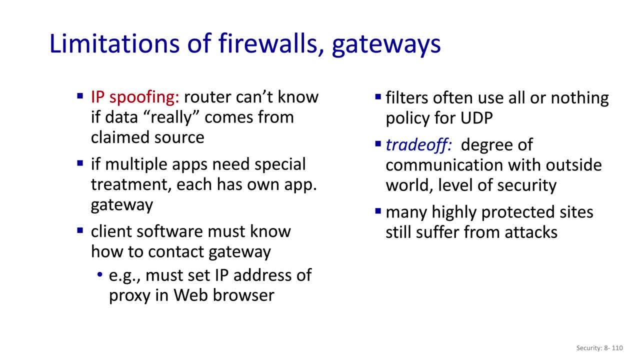 intermediate gateway. The gateway is not transparent. As always, there's trade-offs with the degree of security required and the usability and inconvenience applied to hosts on the network. And even with all of these mechanisms in place, many highly protected sites still suffer from attacks via other vectors. Now we move forward. 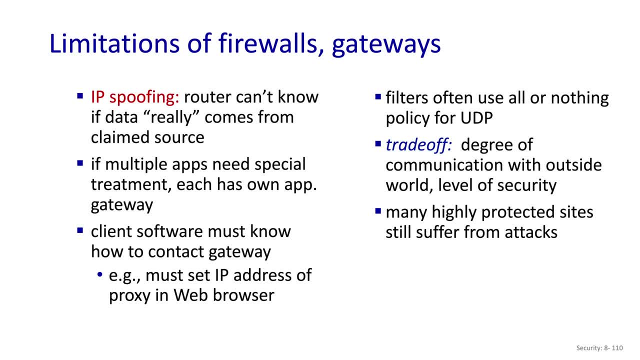 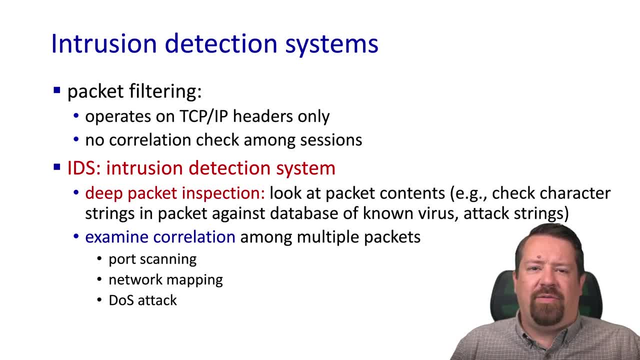 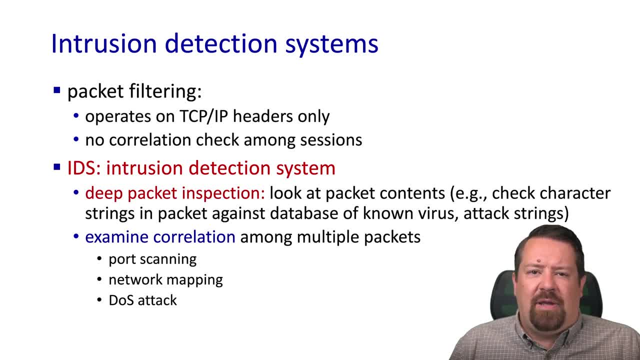 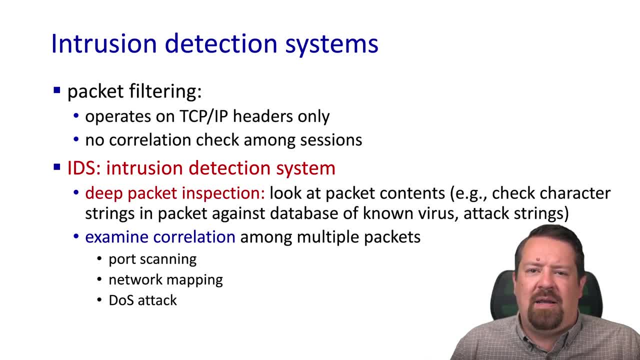 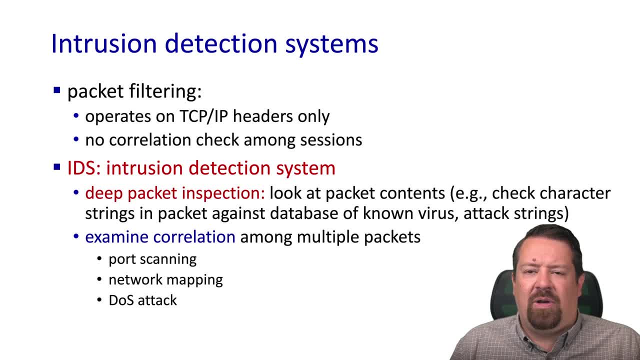 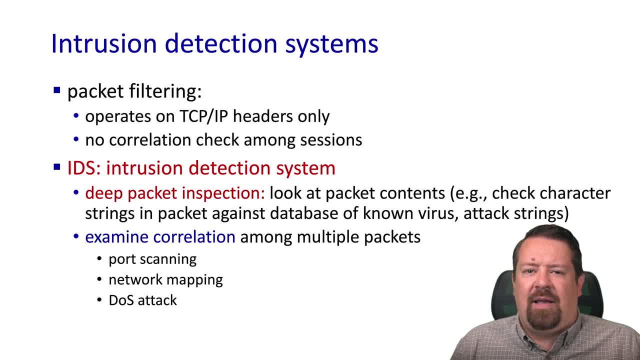 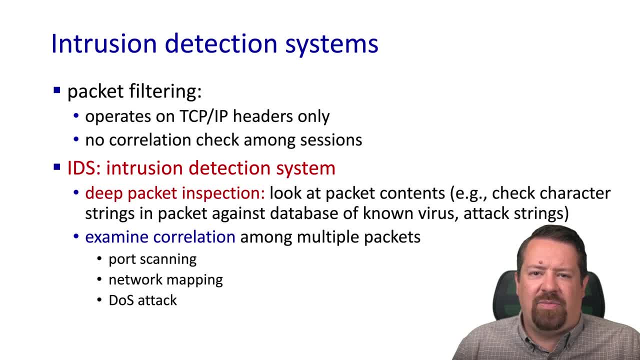 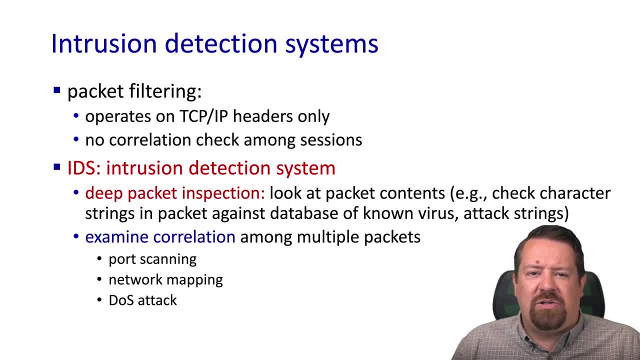 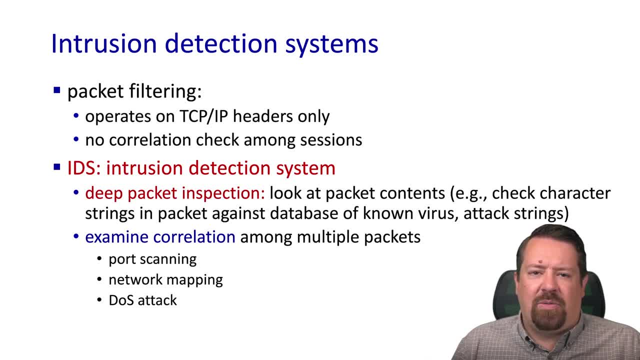 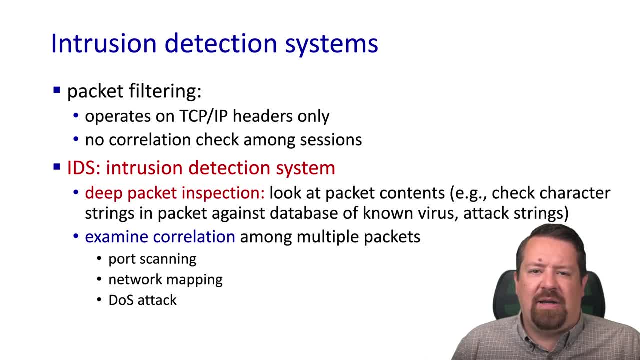 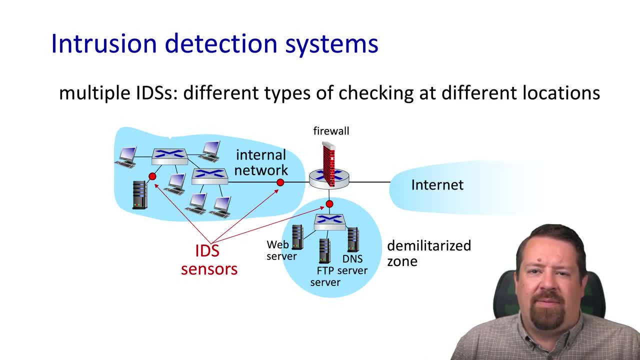 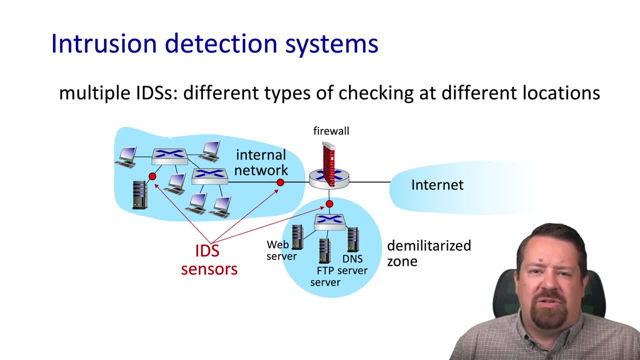 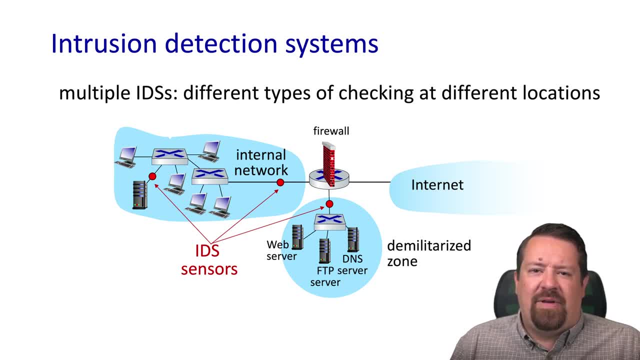